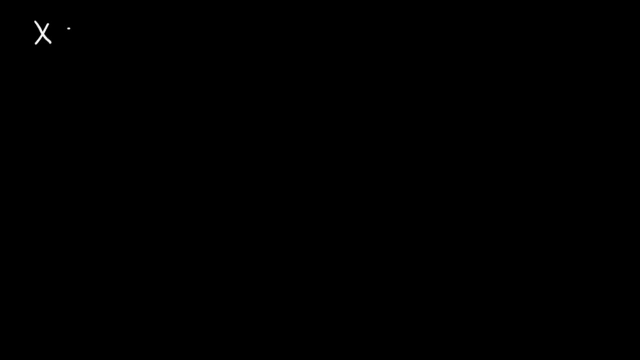 Now how would you graph the equation x is equal to 3? How would you graph that Whenever x is equal to a number, you're going to get a vertical line. So this is a vertical line at 3.. Now, if you think about it, at any point along that line x is always 3.. So at this point we have 3, 0.. Here 3, 2. And here 3, 5.. So x is always 3 in that vertical line. 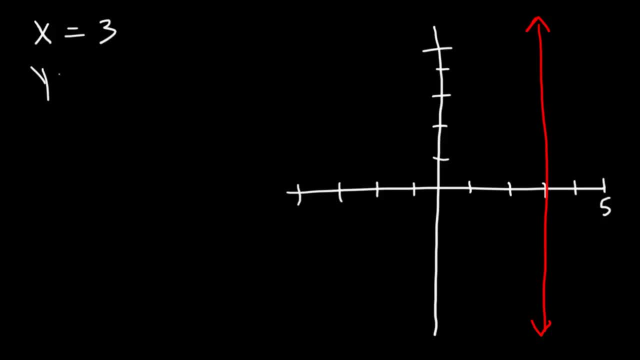 Now what about graphing this equation? Let's say y is equal to 3.. Let's say y is equal to negative 2.. Where's that? Now, if y is equal to a number or a constant, it's going to be a horizontal line. So we're going to have a horizontal line at negative 2.. 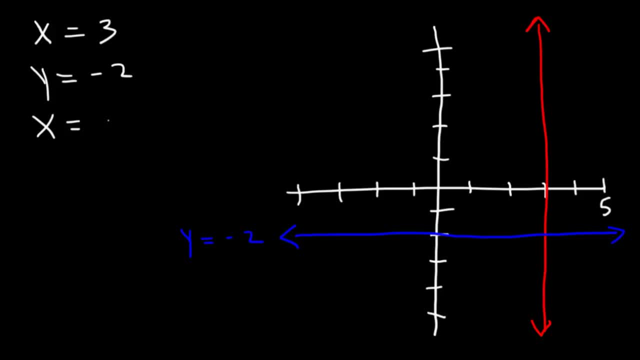 Try these two. Try: x equals negative 3 and y equals 4.. Go ahead and plot those So at negative 3, x equals negative 3.. That's going to be a vertical line, So it looks like that. And the last one, y equals 4.. That's going to be a horizontal line at 4.. 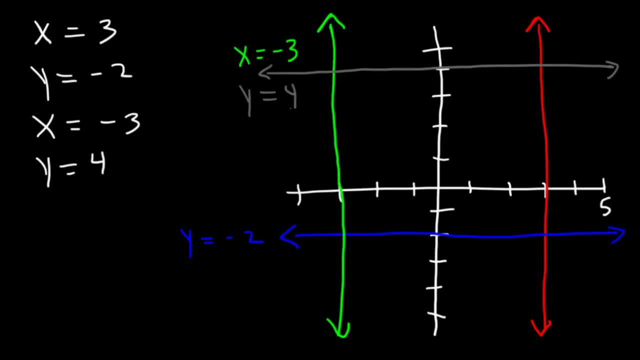 So, just to review, whenever x is equal to a constant, you're going to have a vertical line that goes up and down. Whenever y is equal to a constant, you will have a horizontal line. That's going to be a horizontal line that goes left to right or right to left. 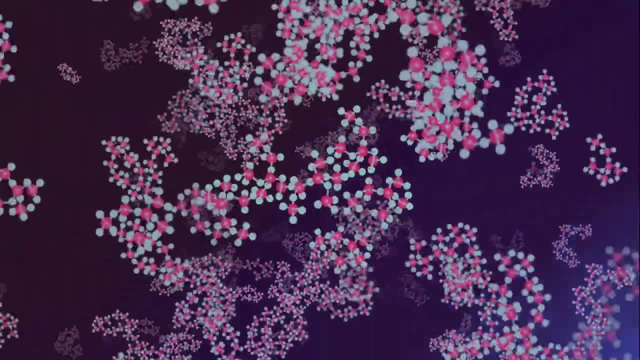 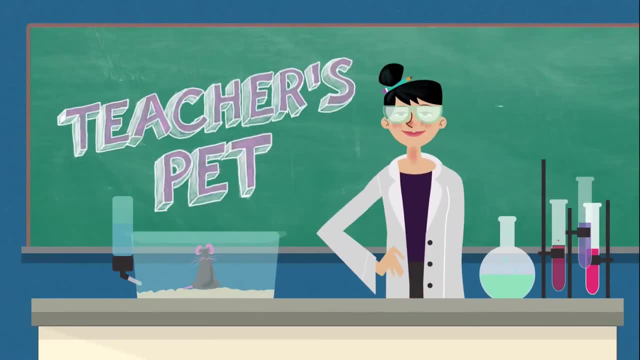 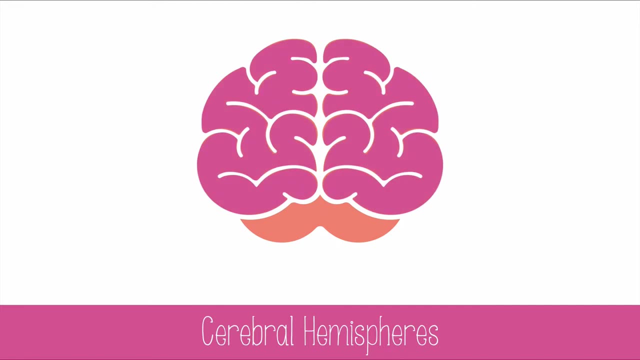 The two cerebral hemispheres process huge amounts of information and are the location of our higher-order thinking. These hemispheres receive sensory input from all the sense organs in the body. The left ear sends sensory information to the left temporal lobe of the brain and